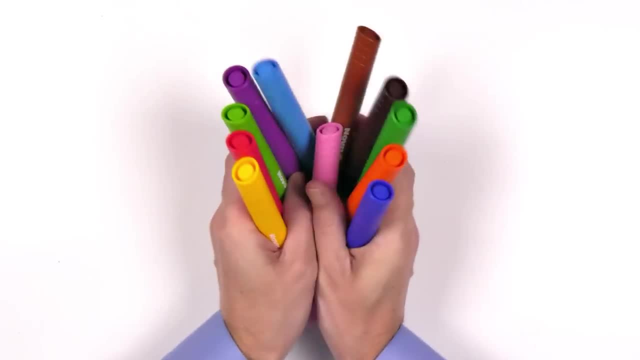 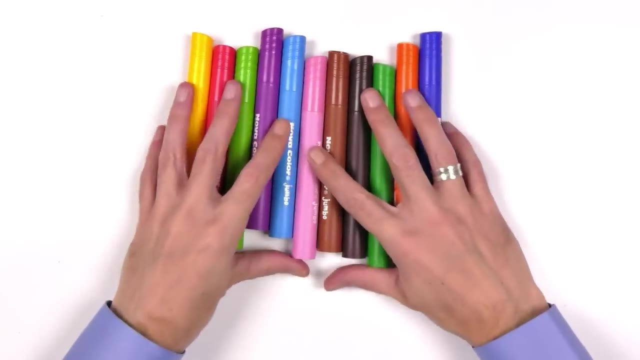 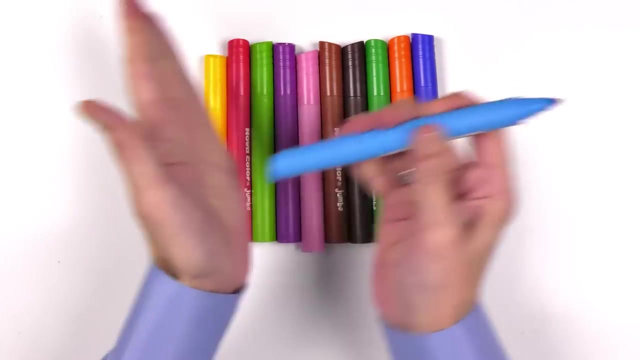 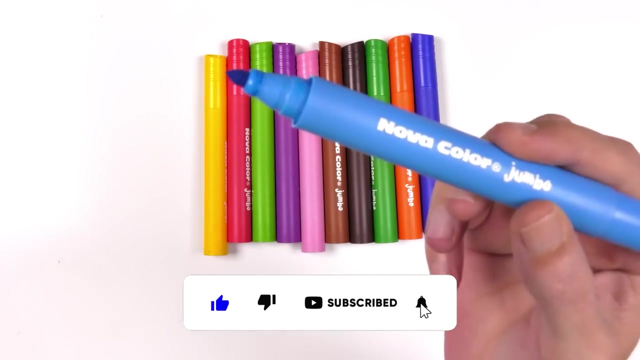 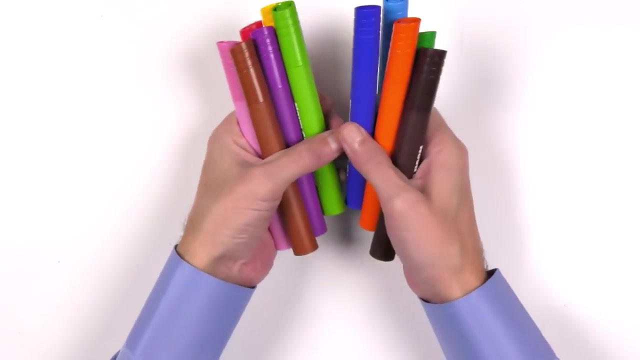 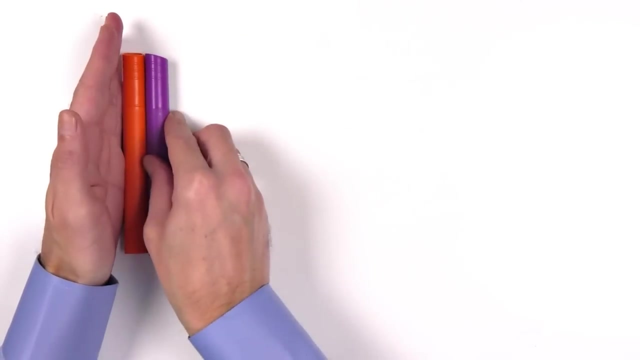 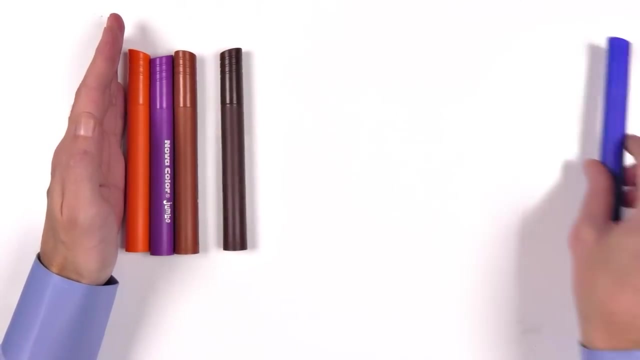 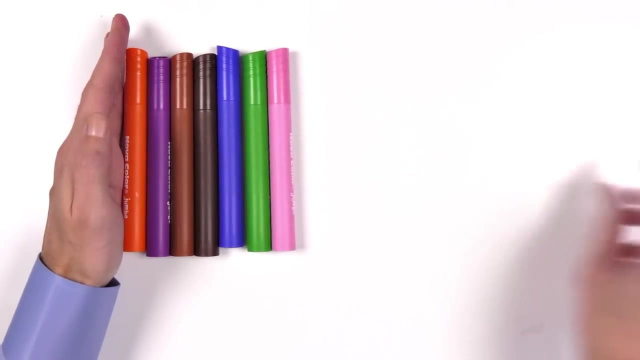 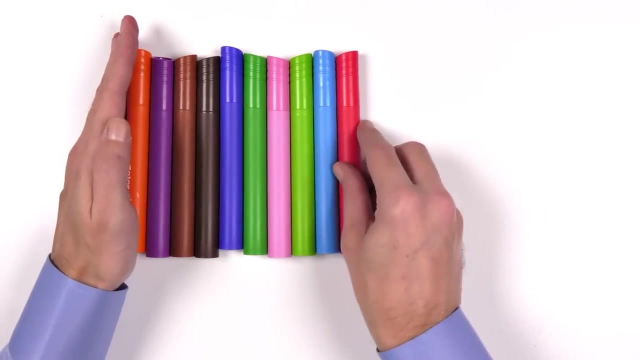 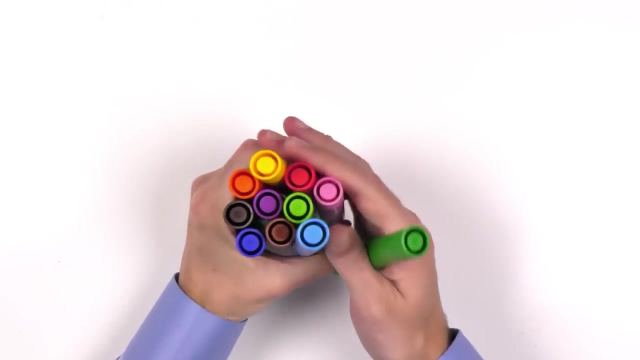 Yes, yes, okay, Wow, it looks great. Congratulations, you're doing awesome. Blue, Wow it looks great. Orange, Purple, Brown, Brown, Blue, green, pink, green, blue, red, yellow. if your crayons could talk, what do you think they would say to you on? 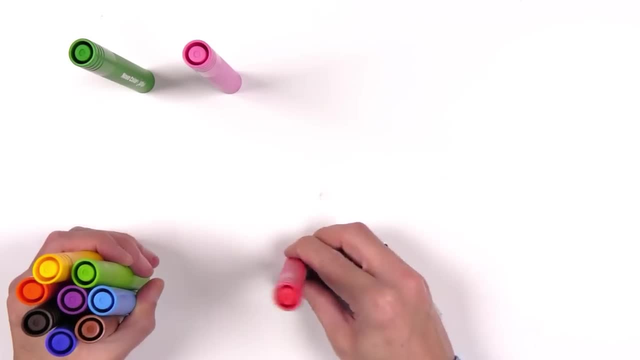 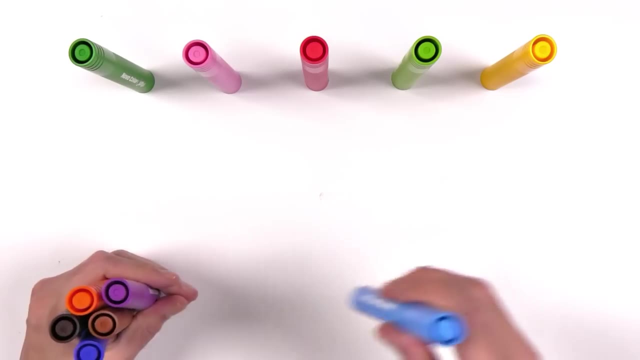 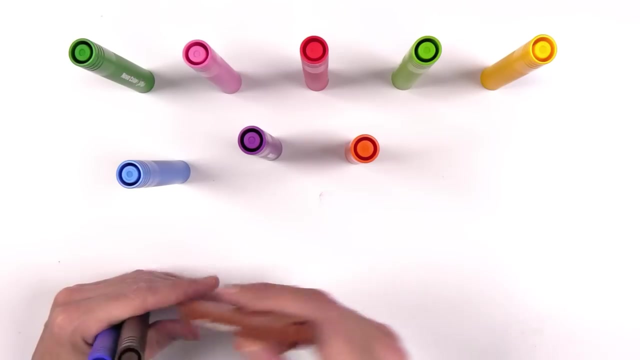 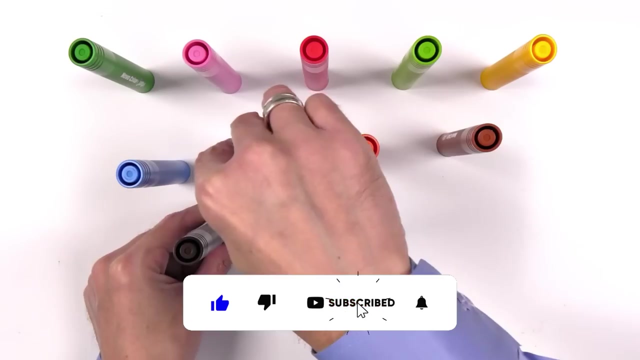 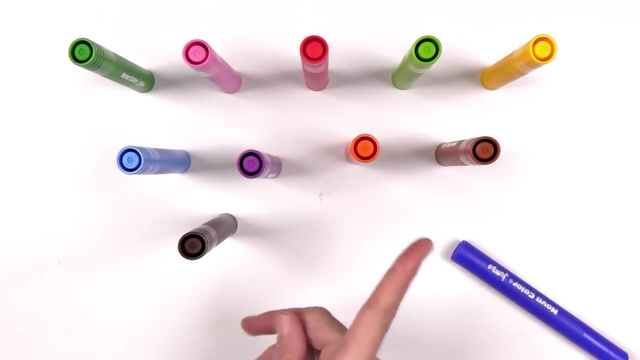 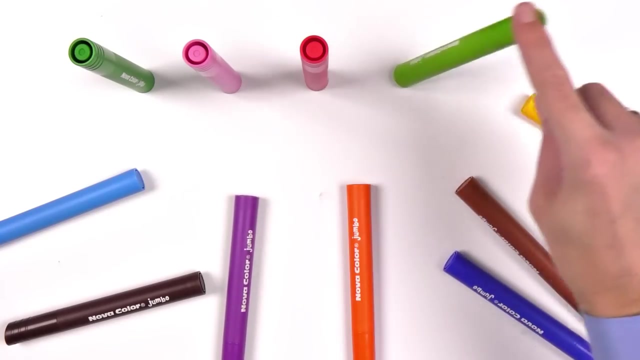 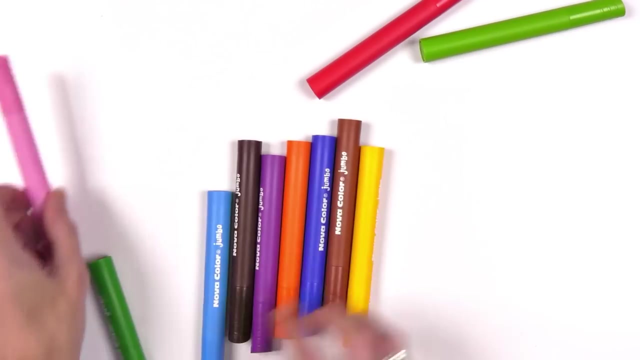 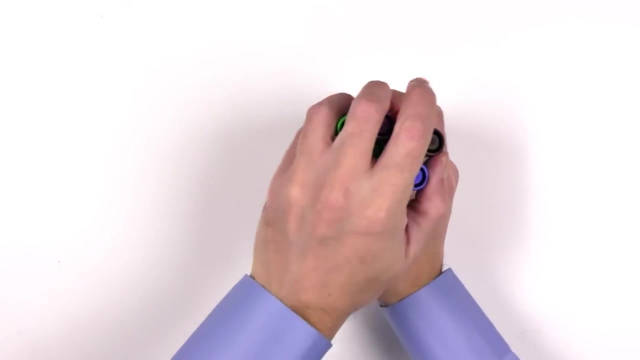 to 3 for 5, 6, 7, 8, 9, 10, 11. if you could draw a magical world, what would it look like? wow, it looks great. do you like messy splattery paintings or do you prefer inside the lines? great, are you ready? let's do it. 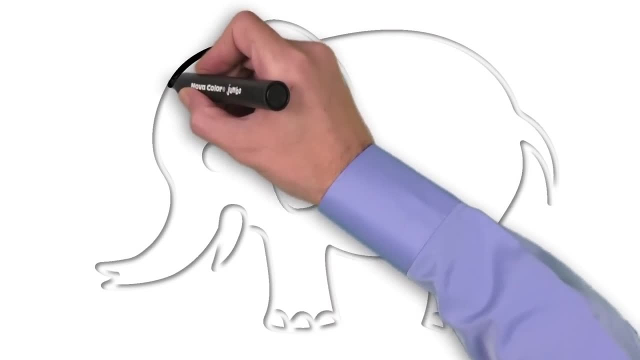 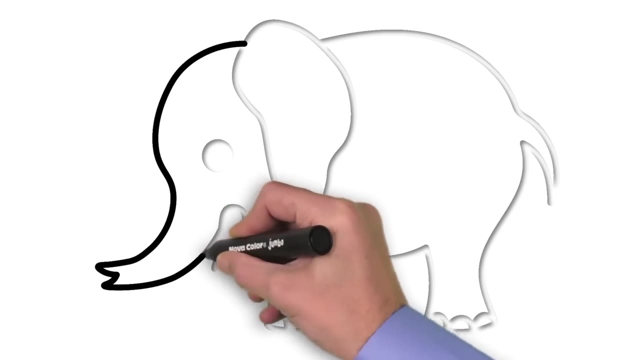 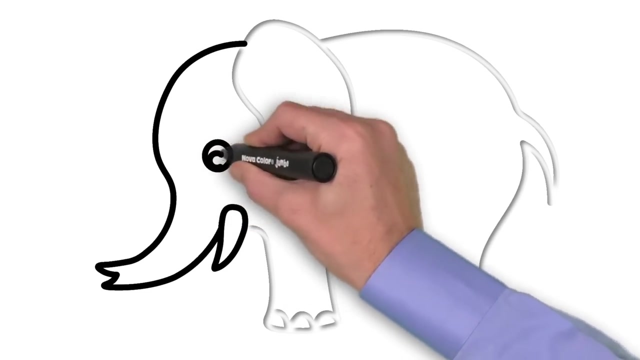 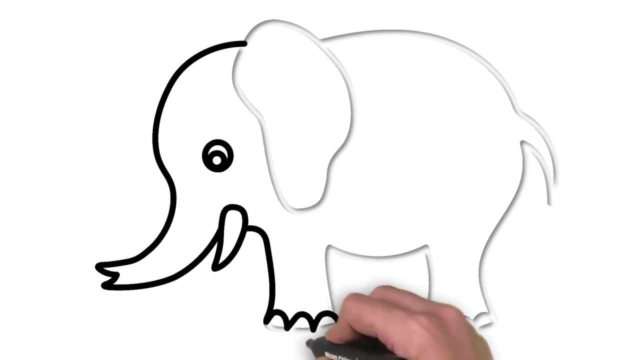 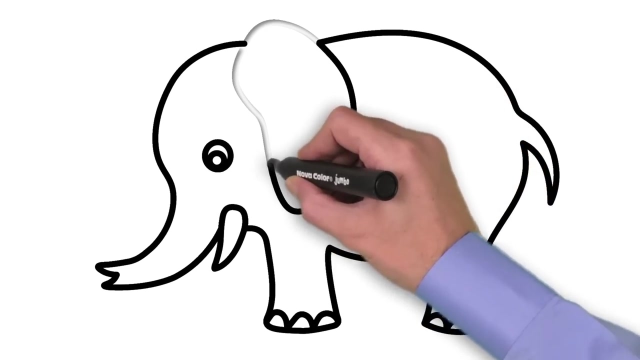 the. now let's dive into the world of thick black pencils. wow, it's fantastic. elephant e is for elephant. an elephant is a big grey animal. it likes to sway its trunk, funded by expert, finished being positive. Wow, it looks great. Feel free to share your colorful thoughts and let your imagination soar. 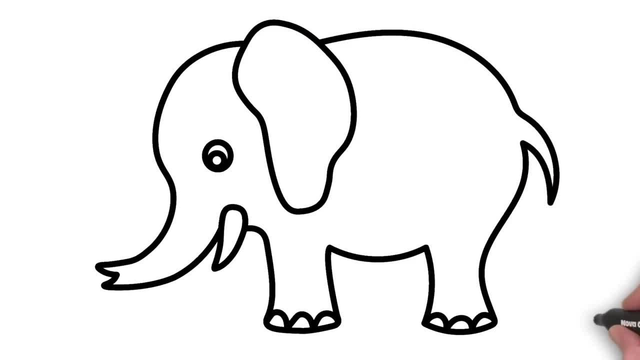 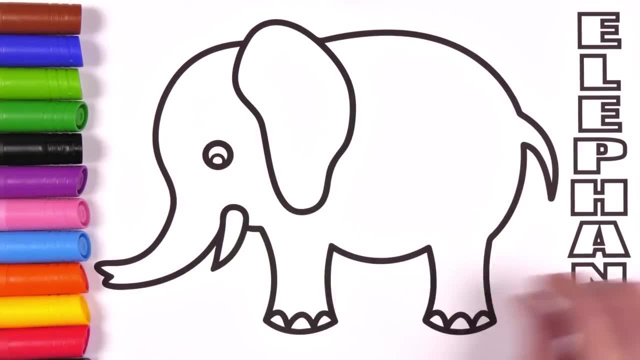 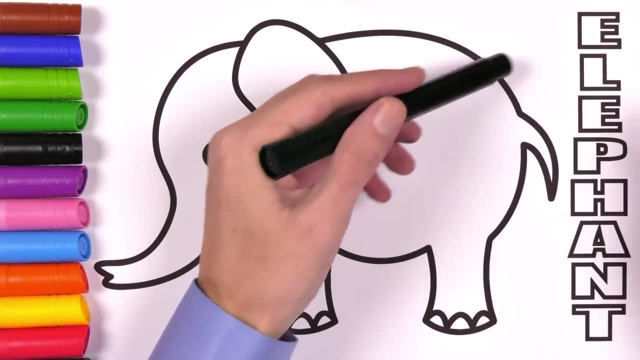 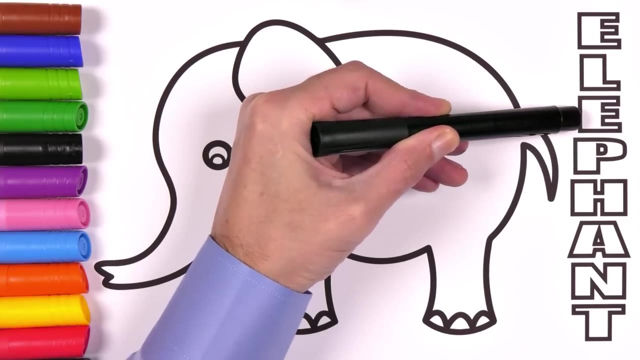 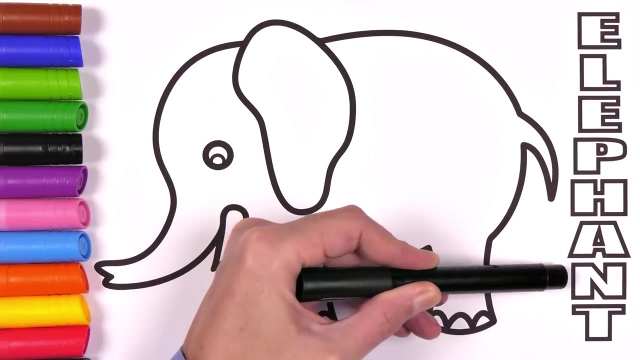 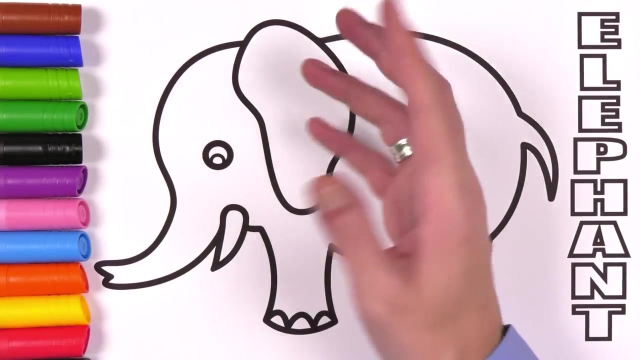 Happy Drawing, Little Friends. Great, are you ready? Yes, yes, okay, Let's do it. E, L, E, P, H, H, E A N T- Elephant- E is for Elephant. An elephant is a big grey animal. it likes to sway it's trunk. 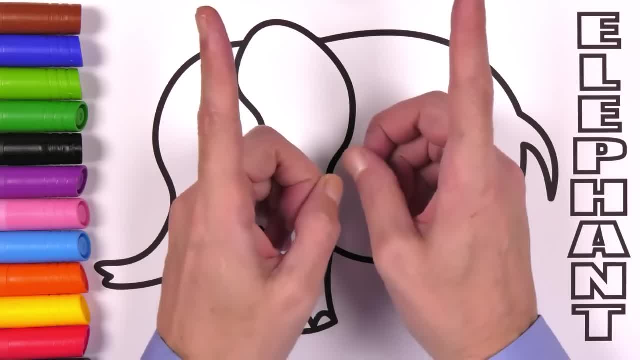 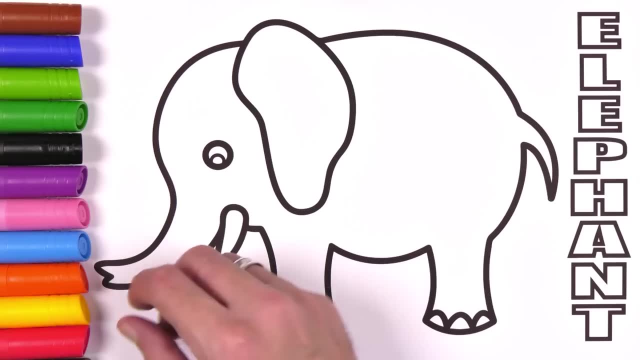 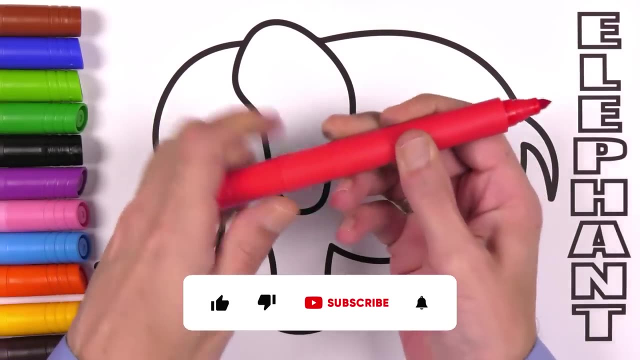 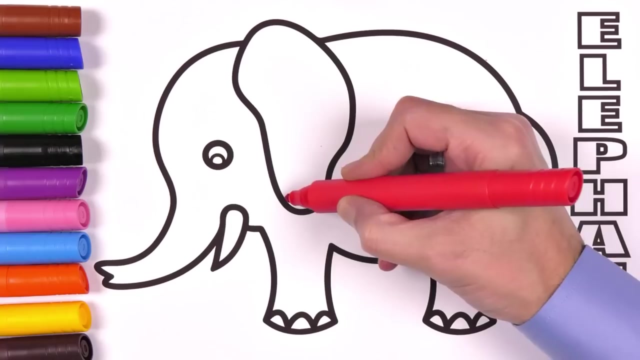 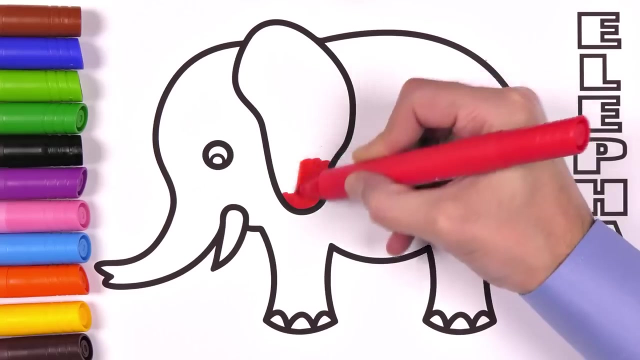 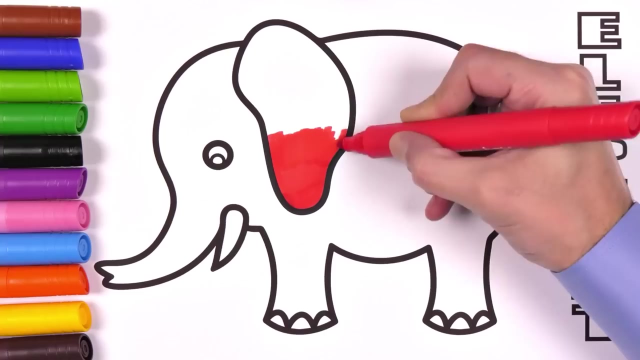 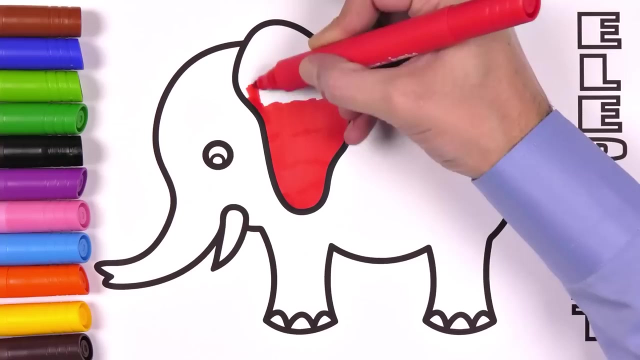 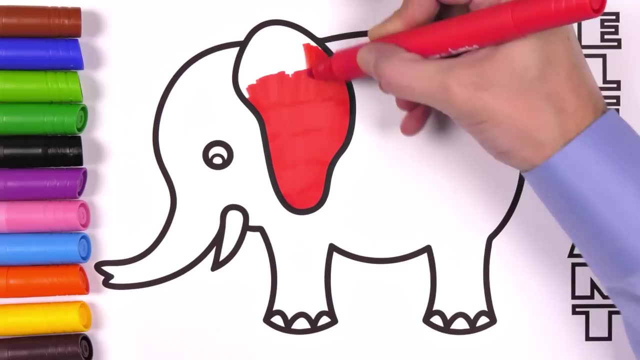 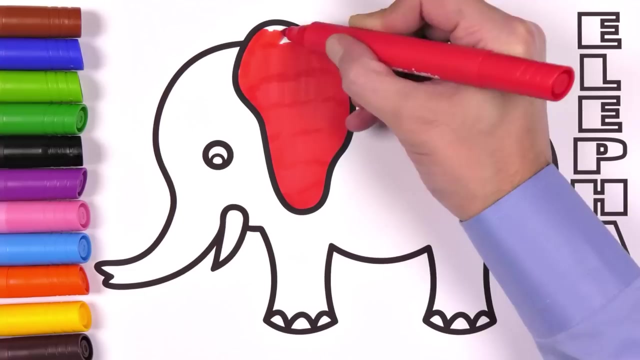 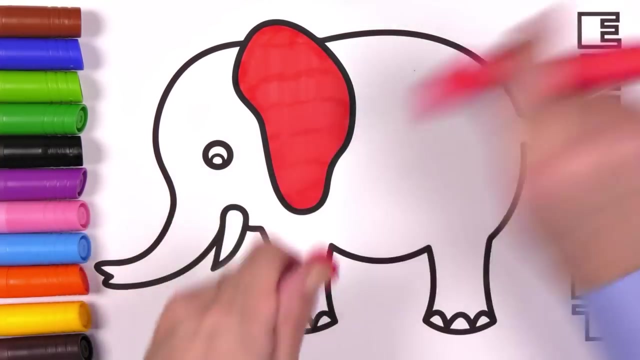 Feel free to share your colorful thoughts and let your imagination soar. Happy Drawing, Little Friends. Let's do it. It's fantastic. Okay, let's explore more colors: red, green, blue and beyond Red. Wow, it looks great. 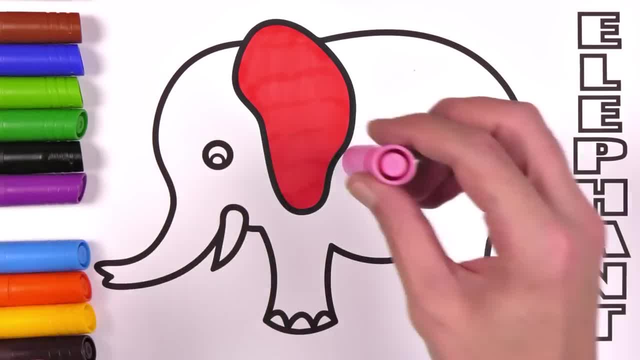 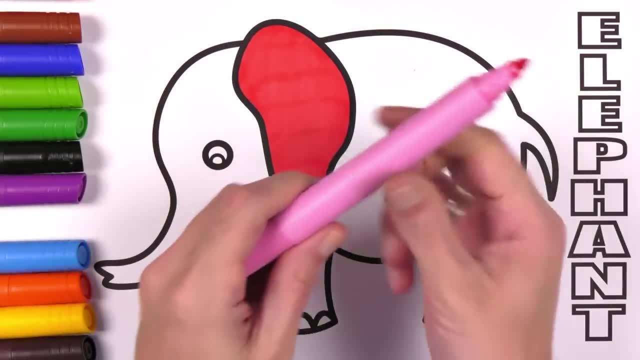 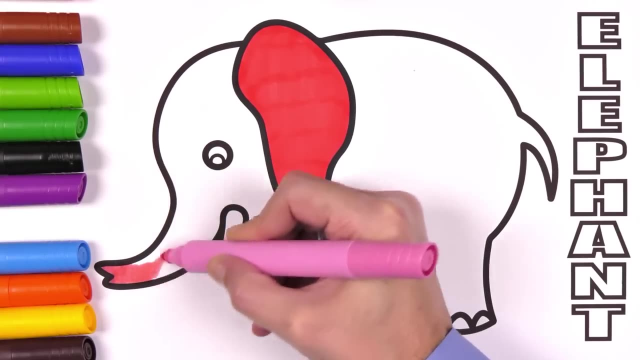 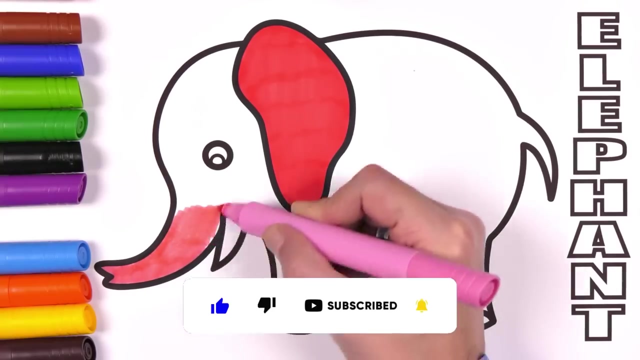 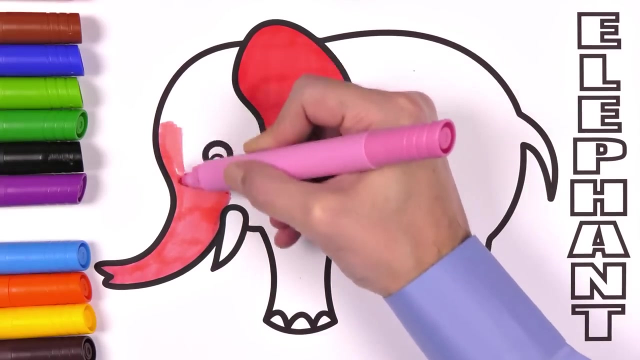 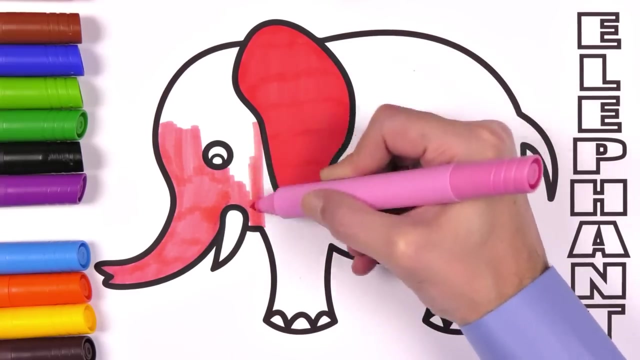 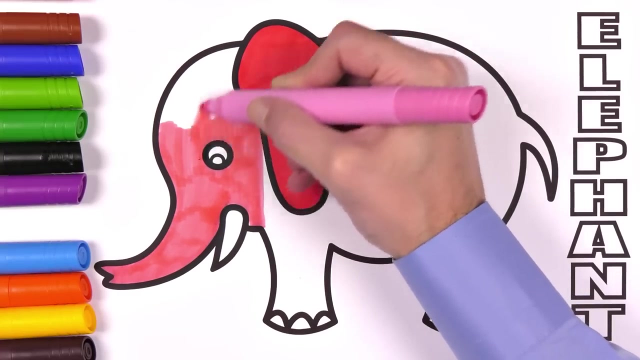 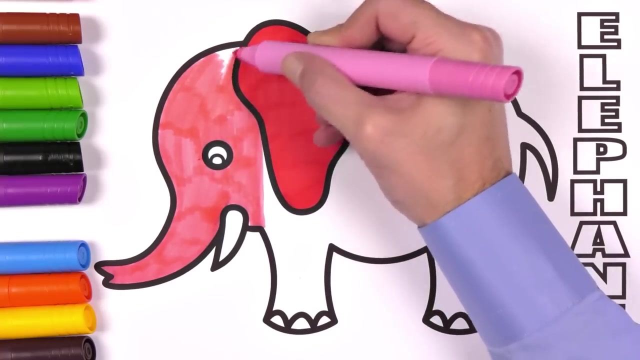 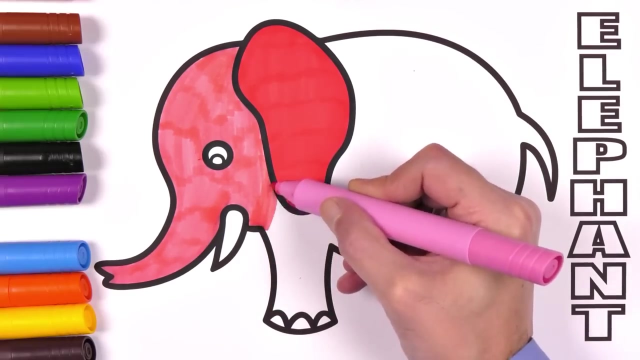 What's your favorite thing to draw? Animals, flowers or something else? Congratulations. Let's create amazing artwork together. Let's create amazing artwork together. Wow, look at these vibrant paints. Join me on a creative journey with playful pens and colorful dreams. 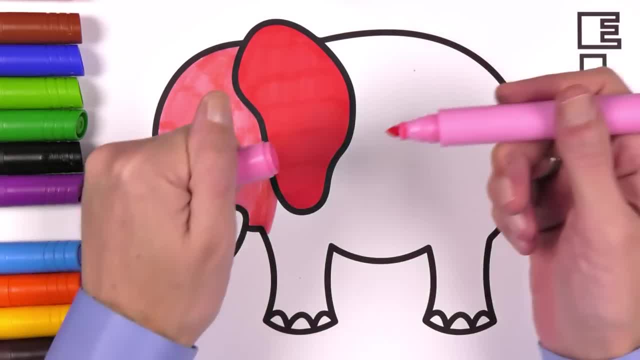 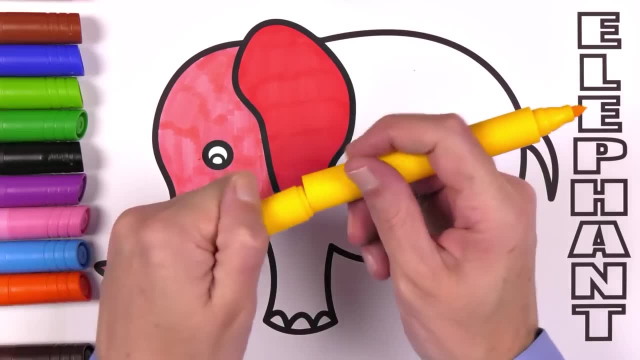 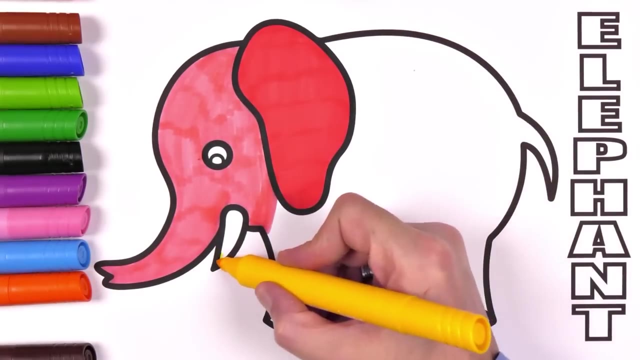 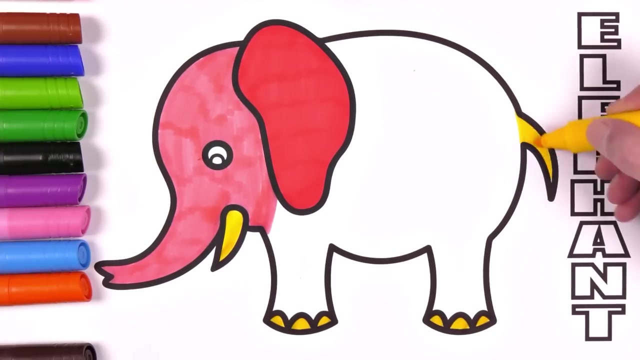 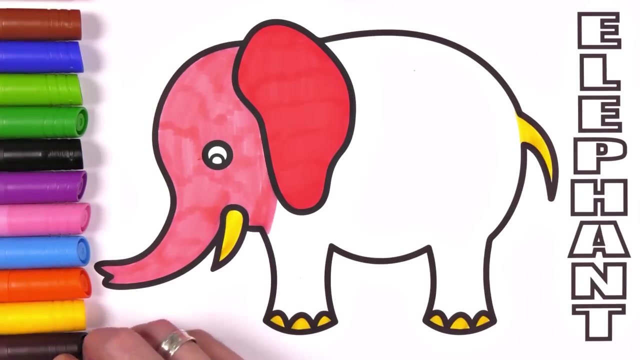 Pink. Do you think your drawings have secret messages that only you can understand? It looks great. Great job. We've got yellow, orange and a rainbow of colors. Let's celebrate with laughter and joy. It's fantastic Yellow. Do you think your drawings come to life when you're not looking? 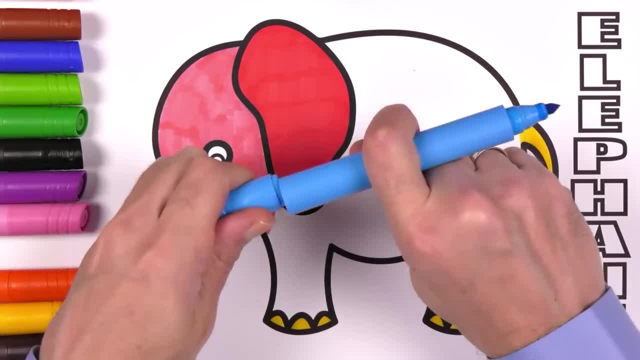 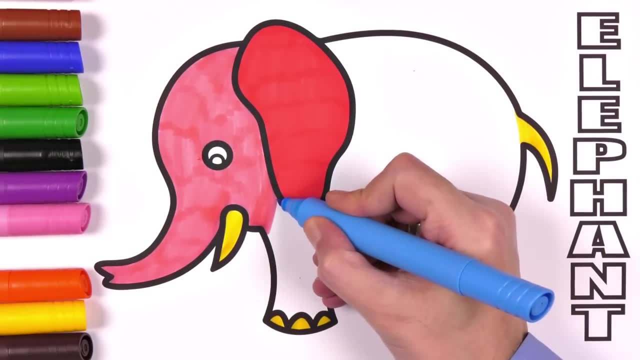 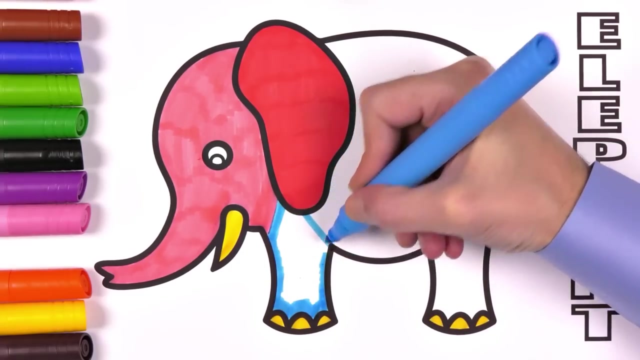 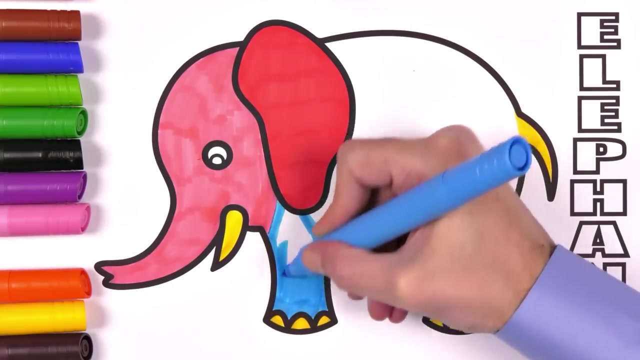 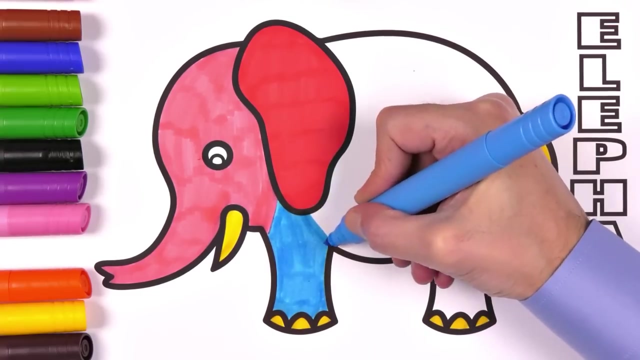 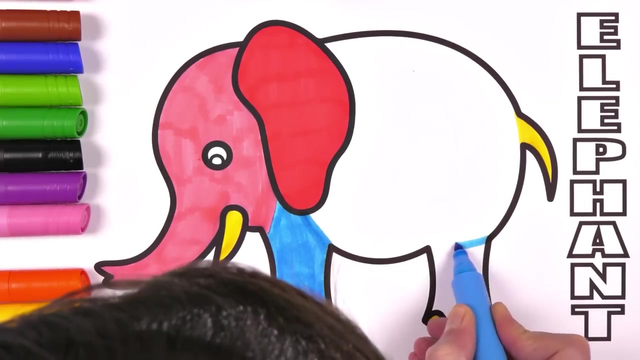 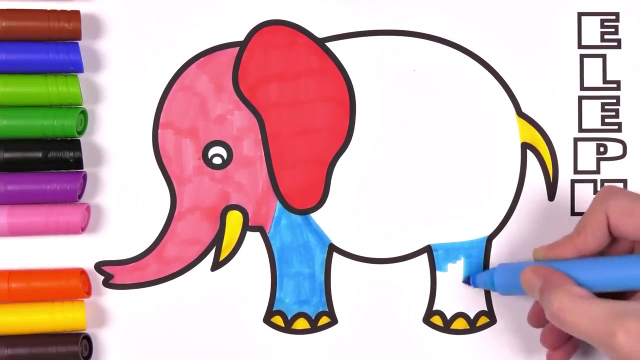 It's fantastic, And I know you will too. Do you think your drawings come to life when you're not looking? It's fantastic. Grab your favorite color. You're welcome together. Guess what color comes next? It's a surprise Blue. If your crayons could talk. 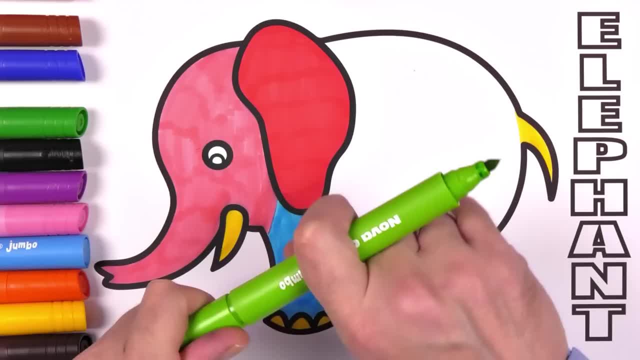 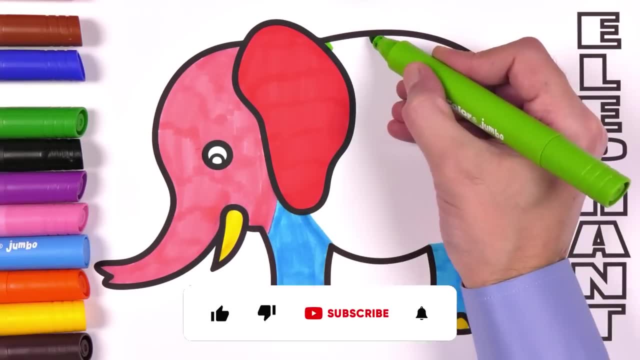 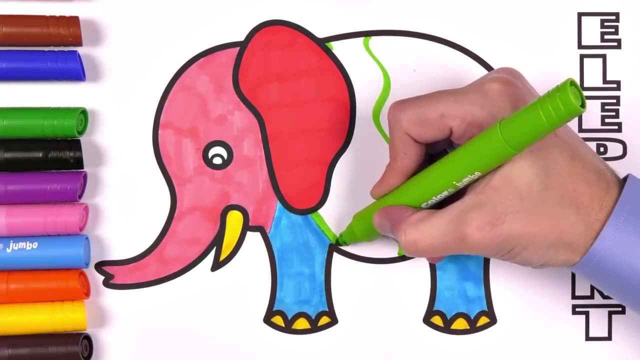 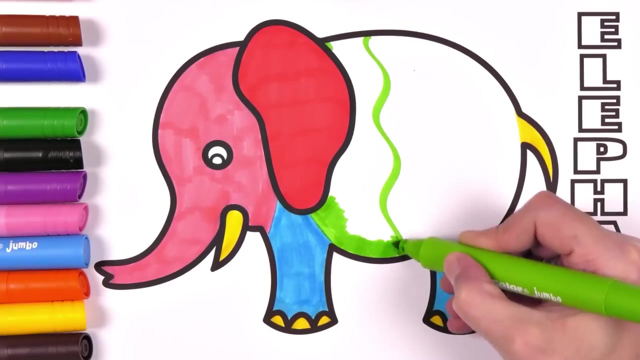 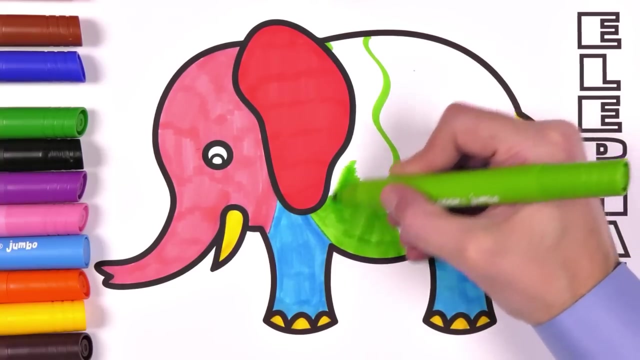 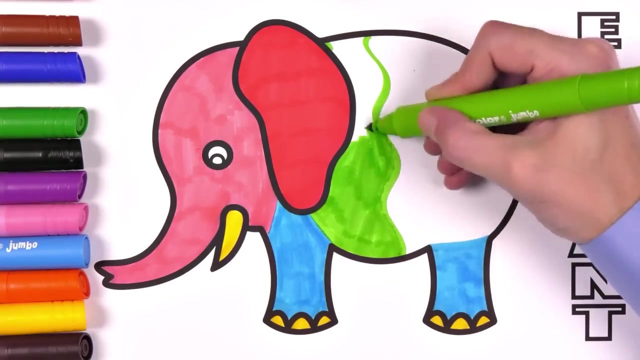 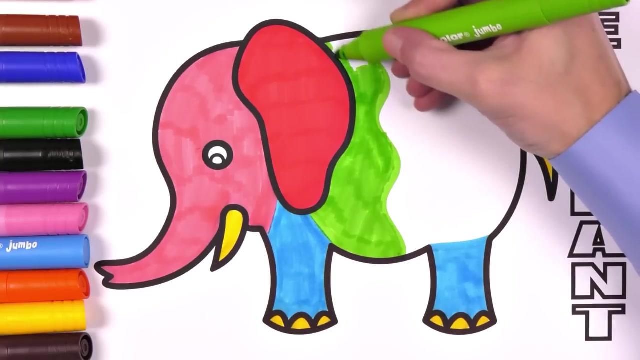 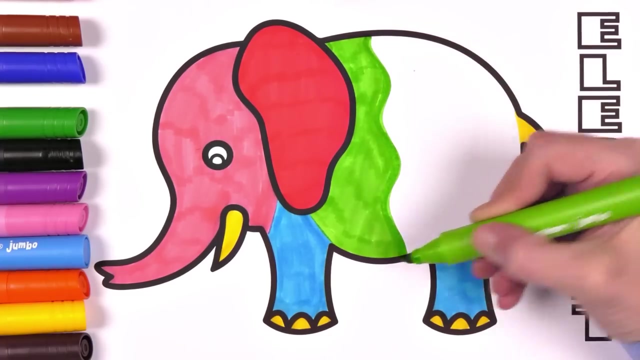 what do you think they would say to you? It's fantastic If your drawings could go on an adventure. where would they go? Congratulations, you're doing awesome. Okay, let's explore more colors: Red, green, blue and beyond Green. 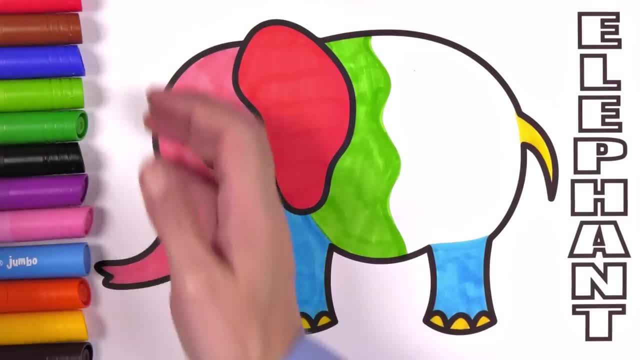 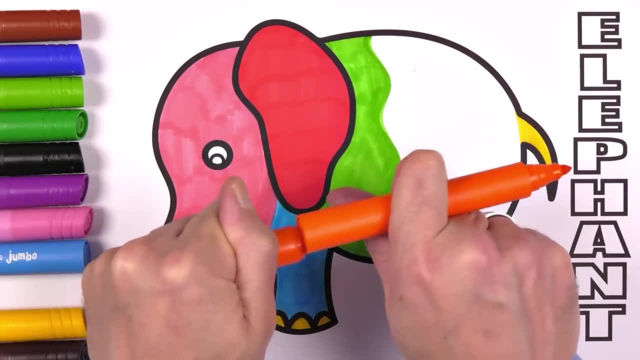 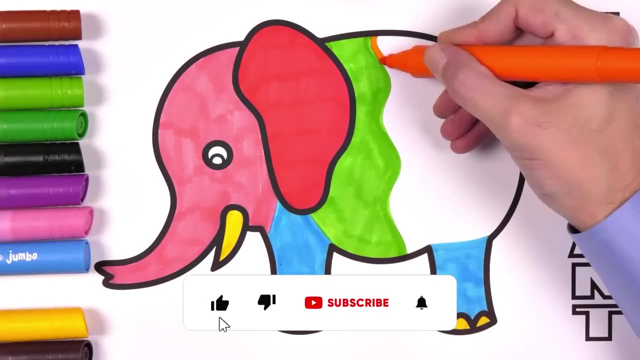 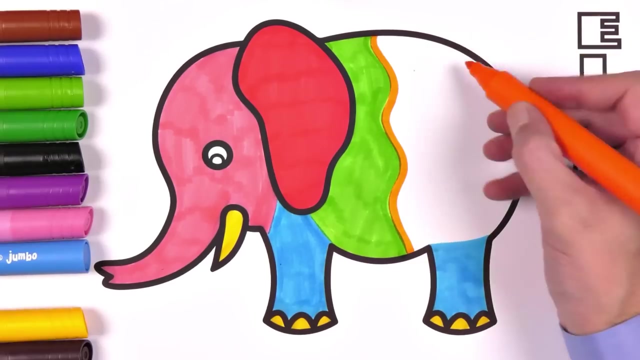 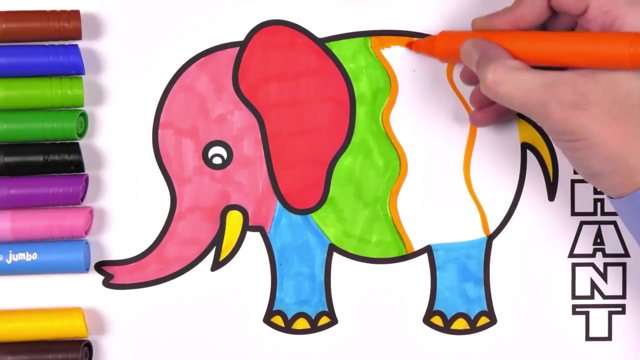 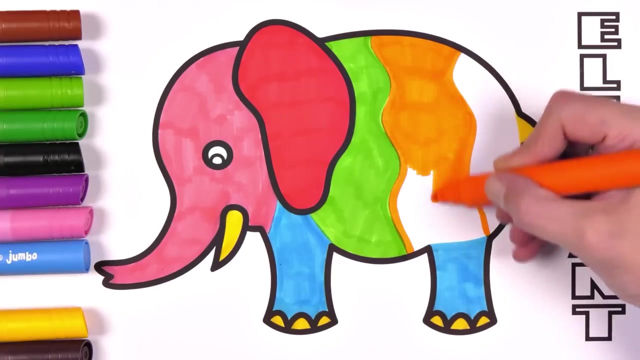 If you could draw a magical world, what would it look like? It's fantastic. Red, green, blue and beyond. Every color. red, green, blue and beyond. Every color tells a unique story. No worries if you're not sure. We're learning and having fun together. 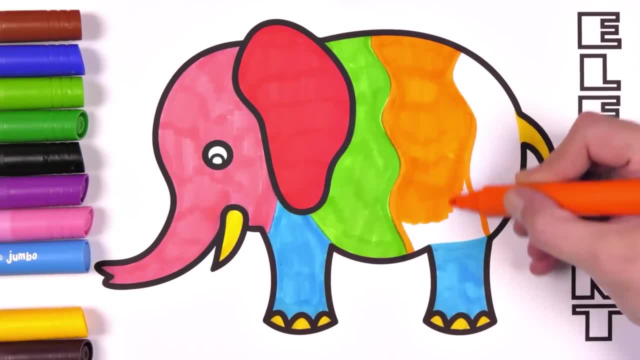 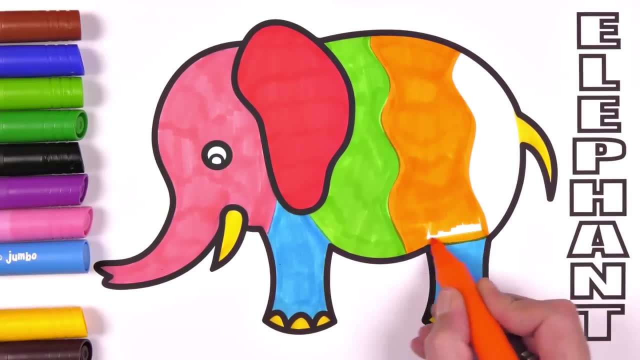 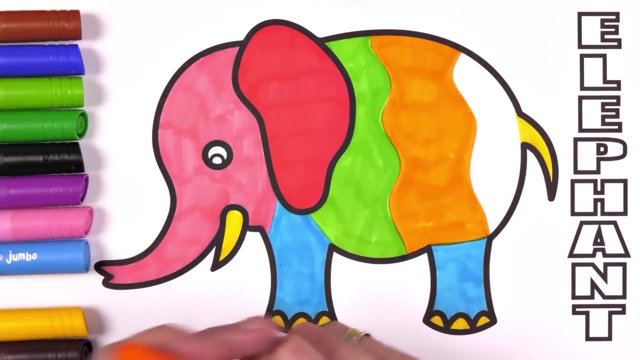 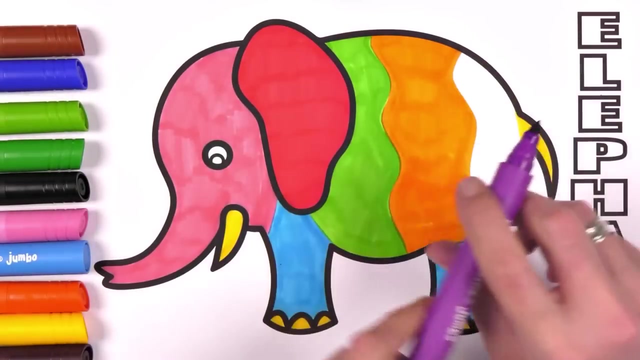 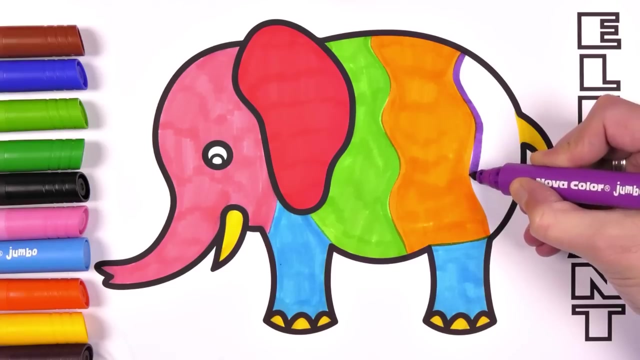 The important thing is to learn and have fun together. The important thing is to enjoy the process. Orange, Which drawing tool is your superhero sidekick? Crayons, colored pencils or markers? It's fantastic. It's fantastic Painting. 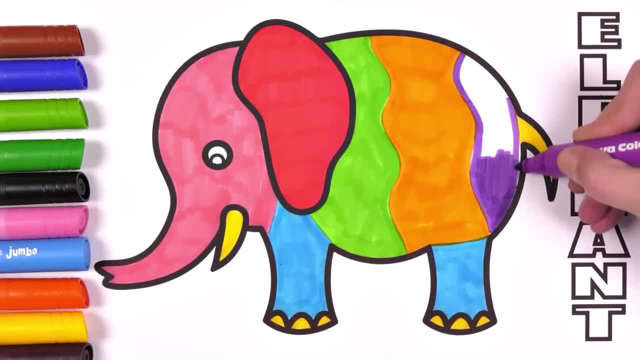 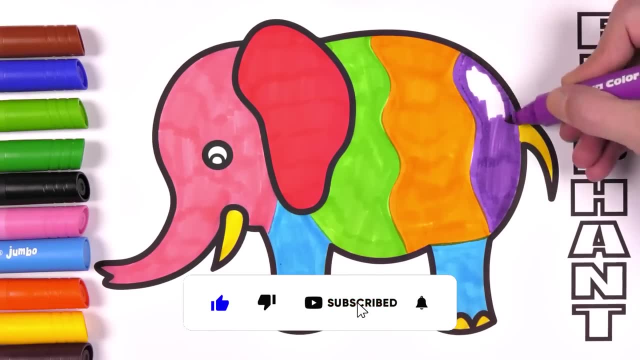 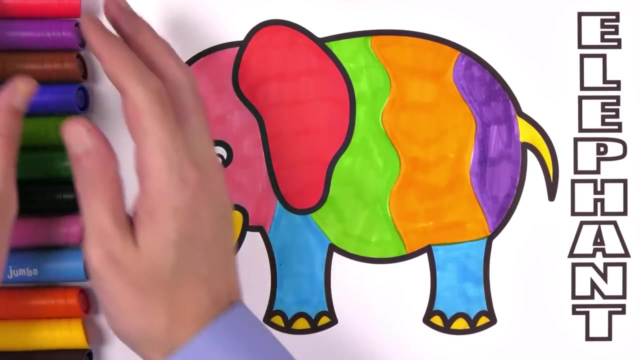 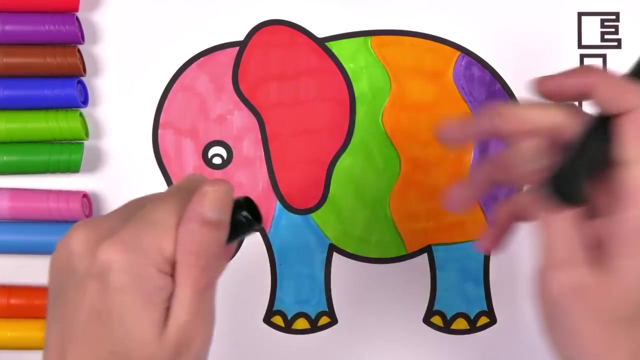 Painting is a wonderful adventure filled with joy. Purple, Purple. Look how they add magic to our masterpiece. Colorful pencils are like magic wands. Look how they add magic to our masterpiece. Colorful pencils are like magic wands in our hands. Now let's dive into the world of thick black. 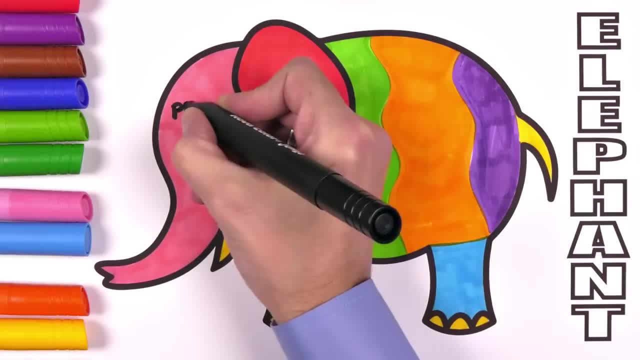 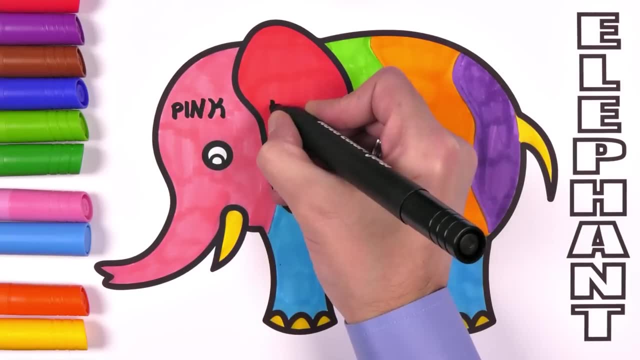 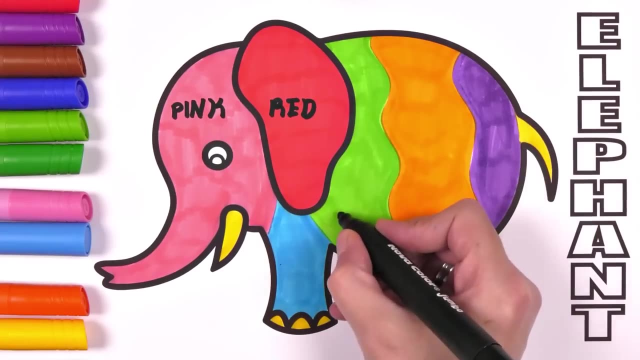 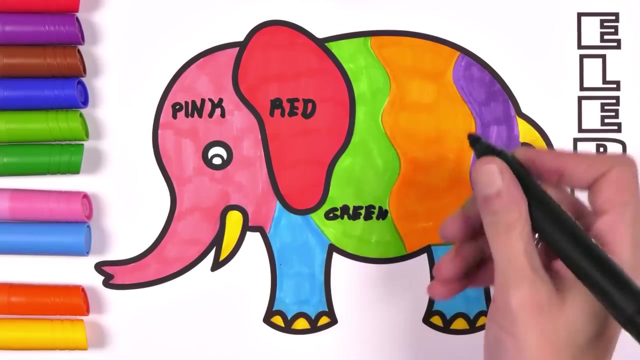 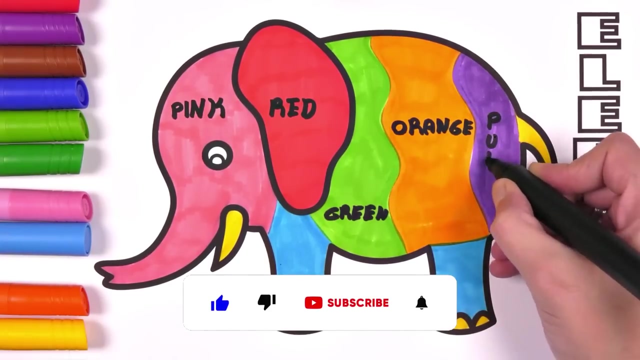 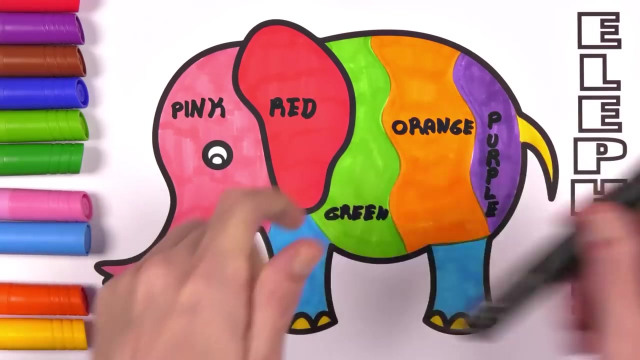 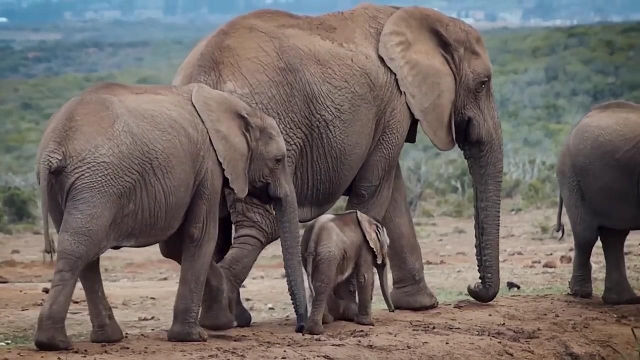 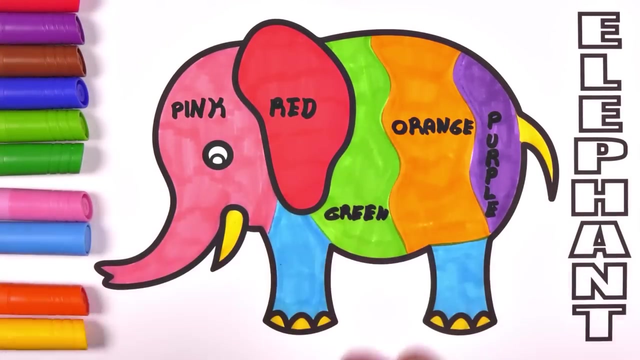 pencils: Pink, Red, Green, Orange, Purple. It's fantastic. Elephant. E is for elephant. An elephant is a big, grey animal. It likes to sway its trunk. Okay, Don't forget to subscribe for more creative adventures. Goodbye for now. 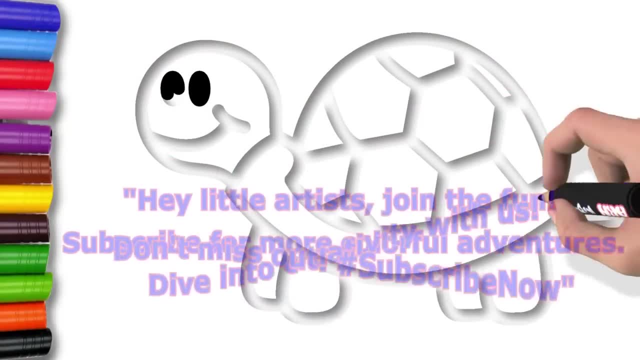 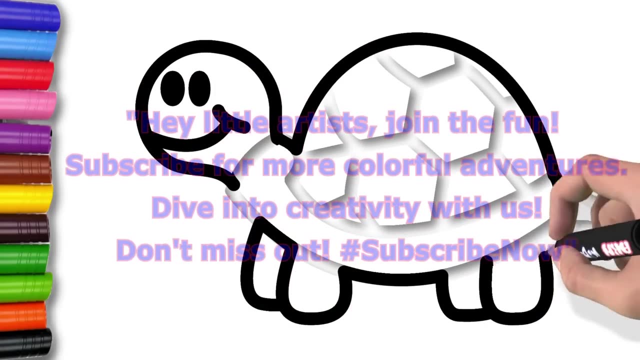 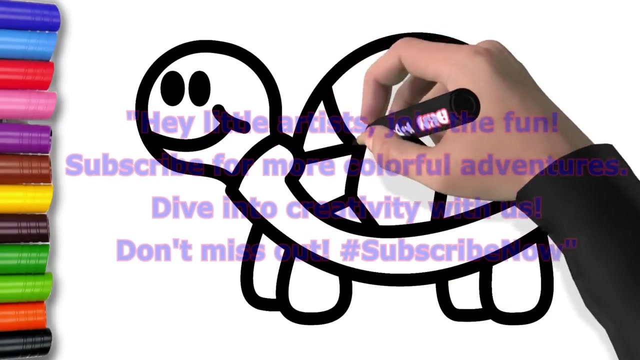 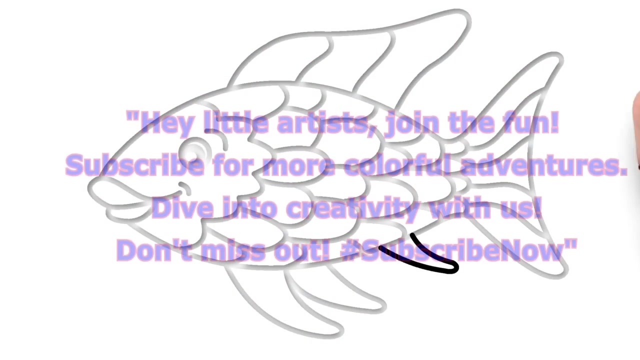 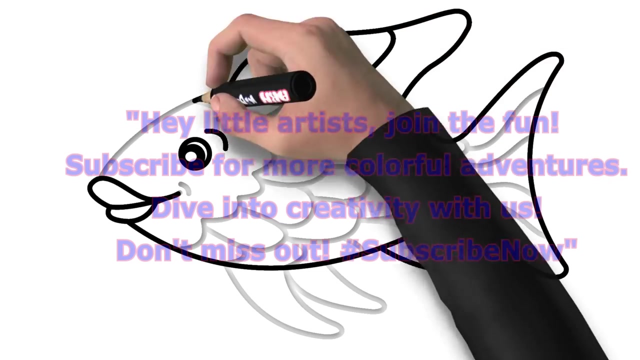 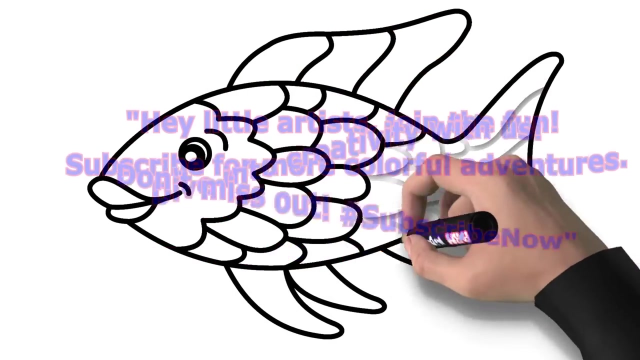 and keep smiling. Turtle T is for turtle. A turtle is slow and steady, always prepared. Fish F is for fish. A fish swims in the sea. Fish come in many beautiful colours In the next videos. goodbye. 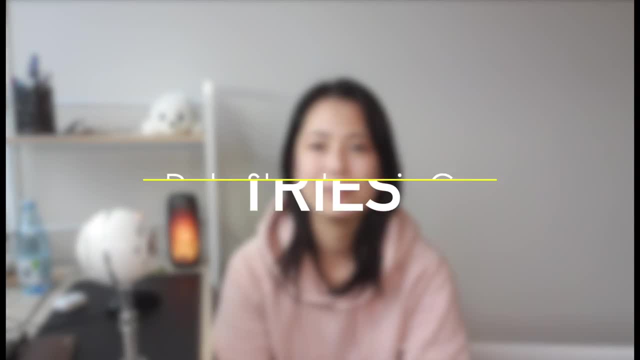 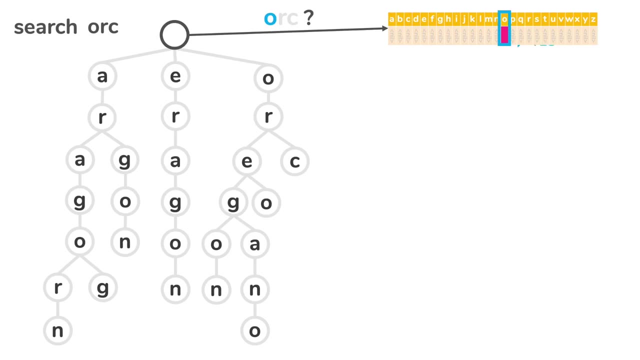 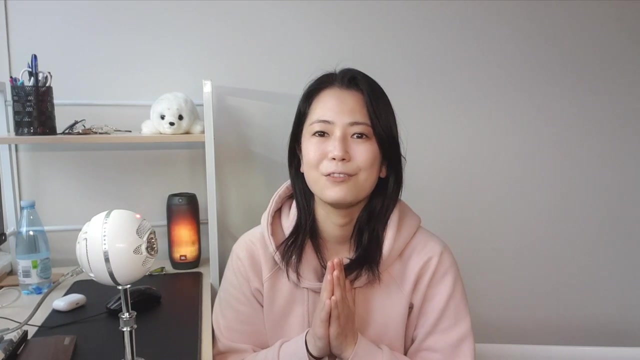 Hello, Today we'll be talking about a data structure called tries. You will learn what tries are and also learn about how they specifically work. Like always, I'll be explaining basic concepts first, with diagrams and stuff, and then after that we will go and do some coding. Okay, so let's dive. 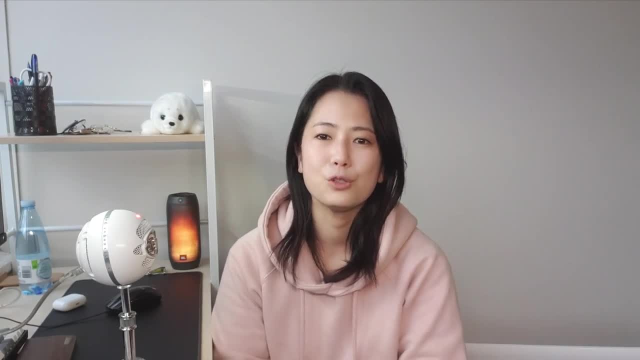 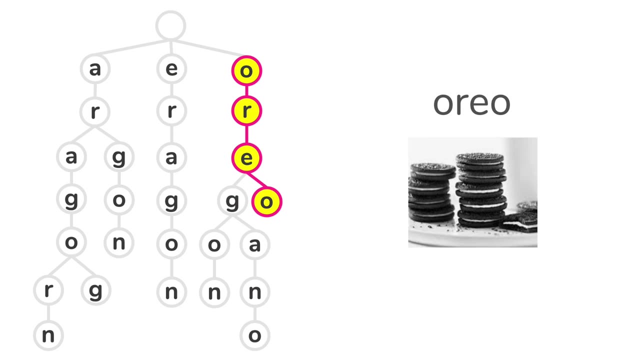 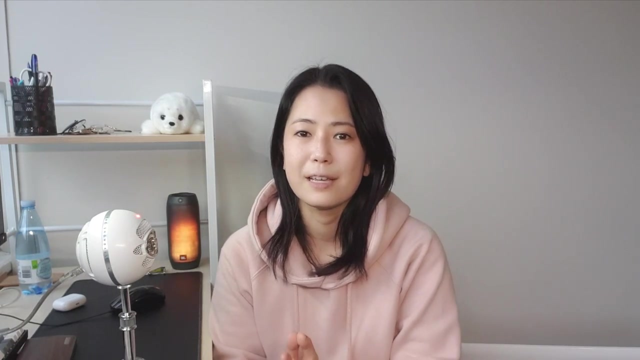 in A try is a tree structure which is mostly used for storing words. Each node will represent a word or part of a word and by connecting the path from the root to that node we can store words in this particular structure. We do this because it lets us search words pretty fast. One application: 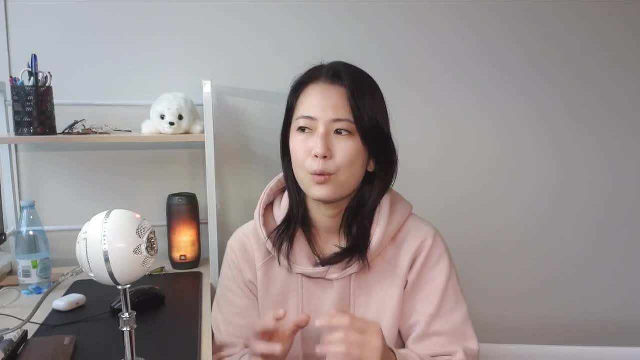 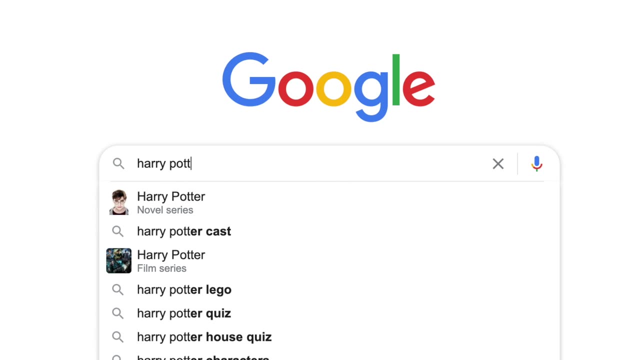 for tries is autocomplete. You know how, like when you're like searching something in Google and as we type in like a search word in the search bar, Google tries to guess what we're trying to type, and the more letters we type in, the more closer it guesses.